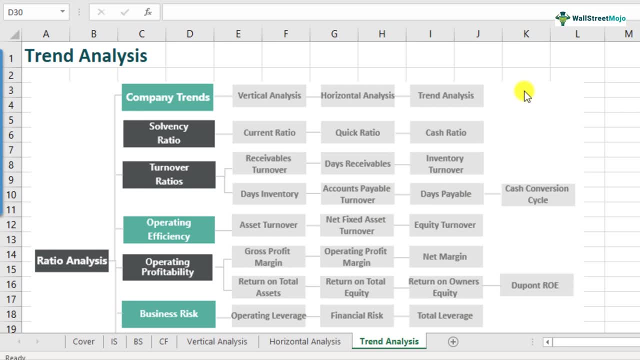 sales or profits or cost numbers within the income statement. You might also want to look at how the trends within the balance sheet items actually look like. Horizontal analysis and trend analysis are pretty much similar in nature. There is a difference in terms of how the base year is. 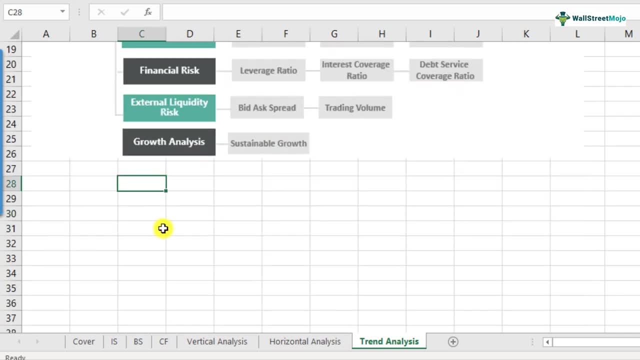 used. Let's discuss this in a bit more detail. I'll take an example here. Let's say: you know, I'll just quickly create some data: Year 2017,, 18,, 19 and 20.. So let's say, we have these four-year data and we have a sales numbers. 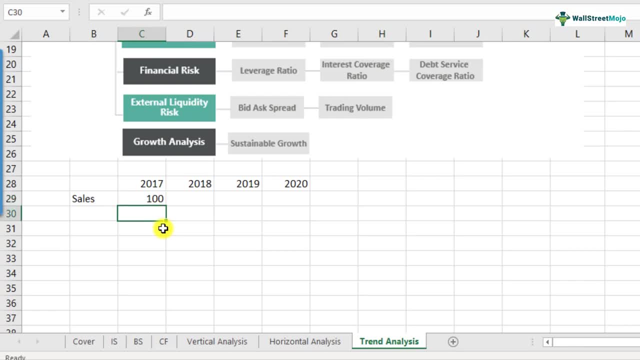 So let's, for the sake of convenience, let's start with sales numbers at 100, 5, 110, 120.. Okay, These are the sales items In horizontal analysis. what we do is percentage growth year over year. So that's what we actually do for horizontal analysis. 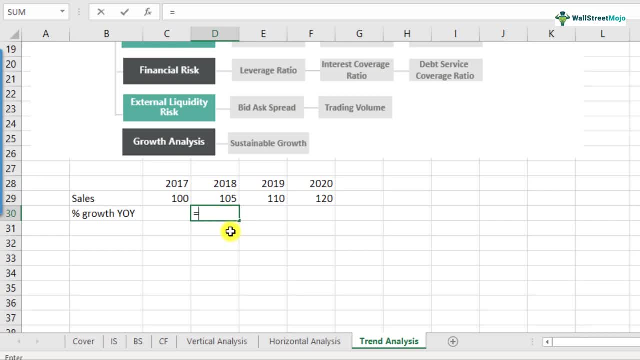 What is the growth rate from 18 to 17?? That would be 105 divided by 100 minus 1.. So this is the formula we discussed in the previous videos, that is 5%. Okay, So this is horizontal analysis I'm discussing right now, So we can see that the 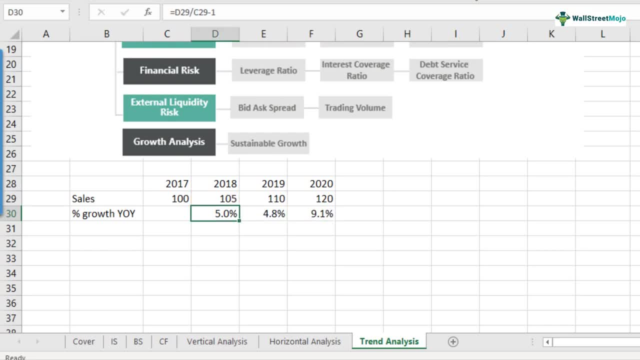 year over year growth rates have is 5%, 4.8%, then 9.3%. When we talk about trend analysis, the key thing here to notice that the base year changes right. The base year for this, 2018, was 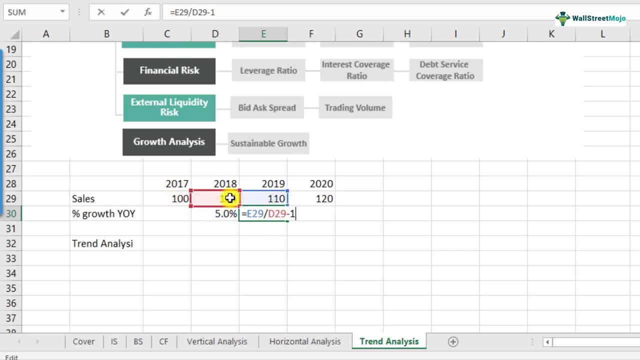 2017.. The base year for 2019 was 2018.. The base year for 2020 was 2019.. As as seen here right In trend analysis, the base year doesn't change. What do I mean by? this is like from the first? 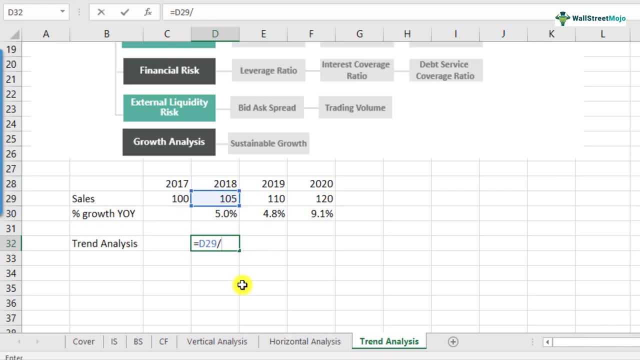 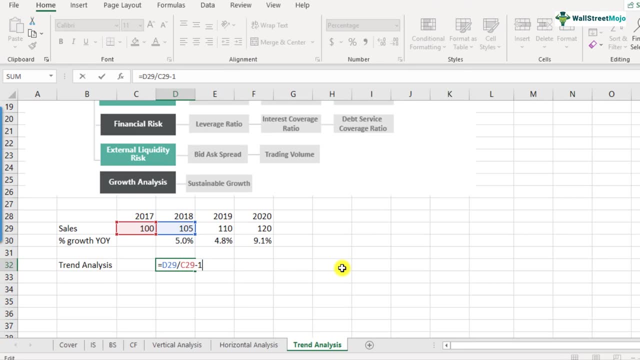 year it is pretty much the same. This divided by 2017 minus one, So that comes out to be 5%. okay, But for the next year- I will not copy. I would have times got 7, or maybe it will come 4%, But I eye. versus my mind. for this trend, I've randomly selected 5%, if I wish to know that that might be because of StoryHelix. right, I did not have a fixed salary, so only that we had $5.5, but it is 5%. 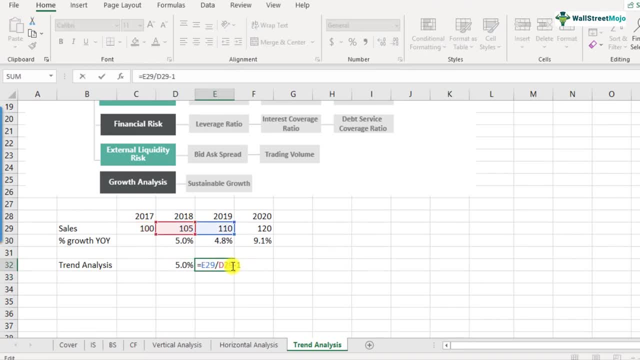 I will not copy and paste this formula: The base year instead of 2018, the base year is actually 2017.. So I'll just shift the base year. So how did 2019 is compared to, you know, 2017.. 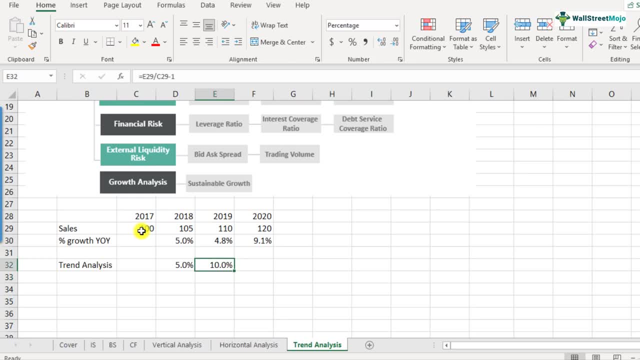 So that's how the trend analysis works. We see that there has been a 10% growth over a two year period- right. Likewise, we do the same for 2020.. Again, I'll shift the base year to the 2017.. 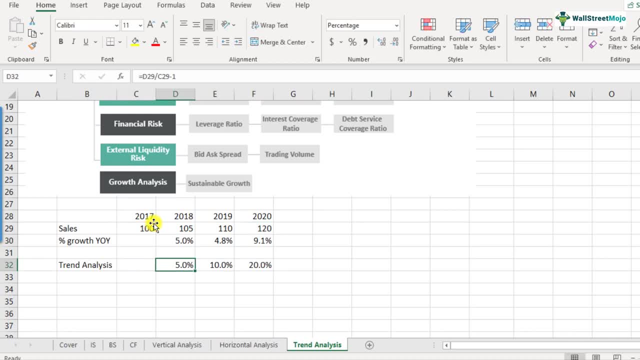 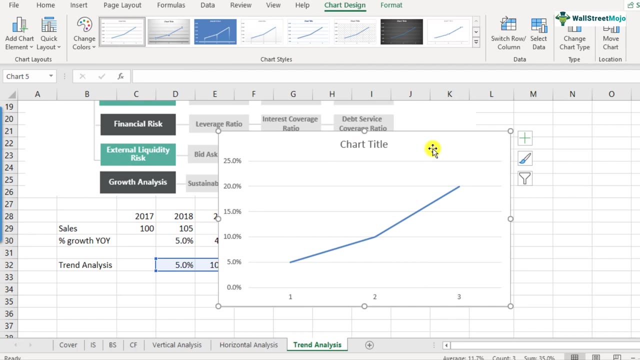 So what do we note here is that the trend analysis takes the base year as 2017 only, and it doesn't change. okay, And usually this can be plotted on a graph to probably understand this in much more detail. Usually a 2D graph can be used for this. 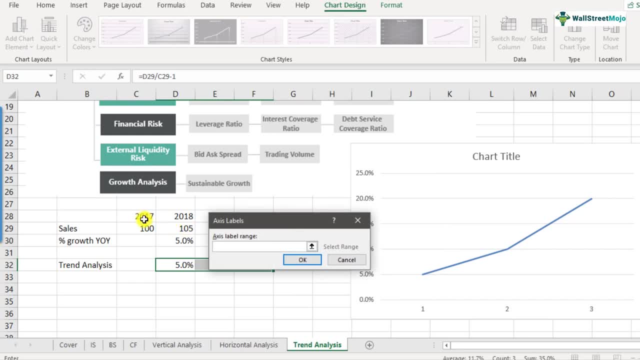 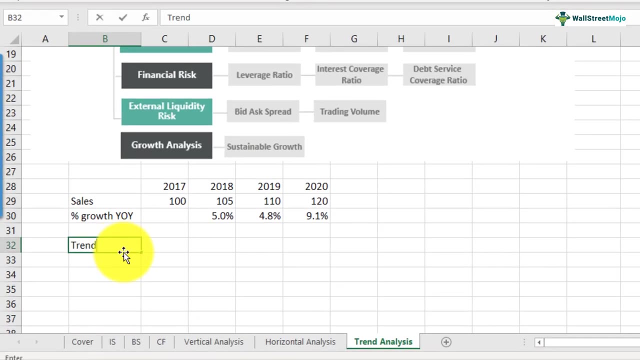 And let me just change This data as well: for years, As you can see, for 2017, there was a 5% growth- 2018, you know, as compared to the foundation year that is 2017.. So when we look at the trend analysis, basically the base year doesn't change. 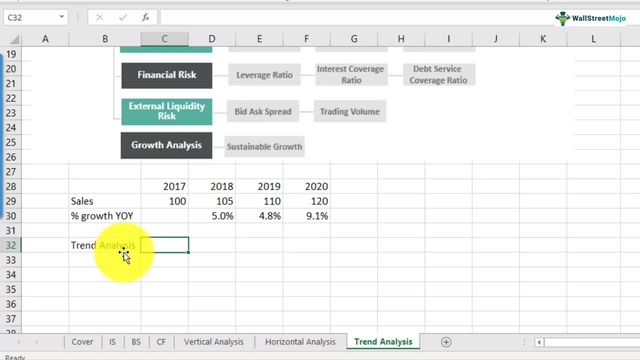 It remains at 2017 itself. So the first year, what we do here is we take this like 100 divided by 100. So it comes as a hundred percent. Okay, The next year would be 105 divided by the base year. that comes out to be 105%. 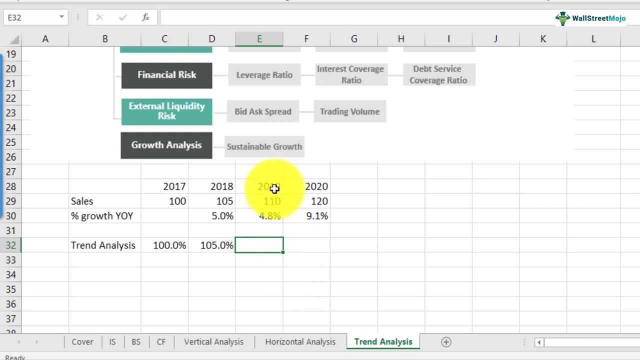 The next year, 2019, will not be compared to 2018.. It will be compared with 2017 itself. So we will use 110 divided by 100.. So the base year is not shifting here, as you can see, right. 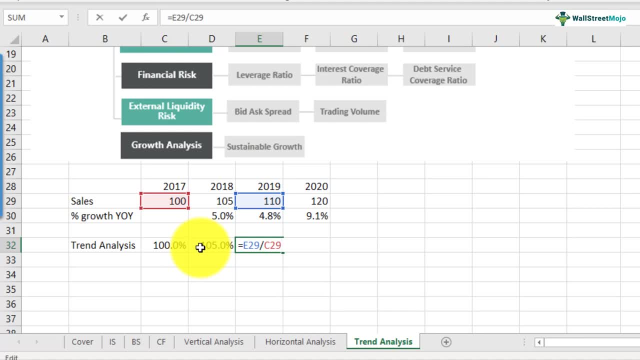 It's the same for all the years, Likewise for 2020, it will be the same. Okay, So it will be 120 divided by 100.. As you can see here, the trend analysis also gives us a trend as to how sales have moved. 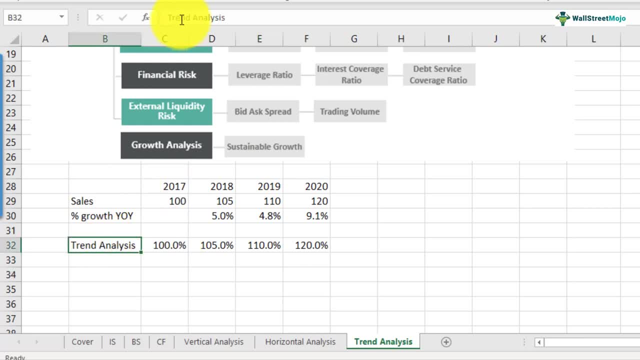 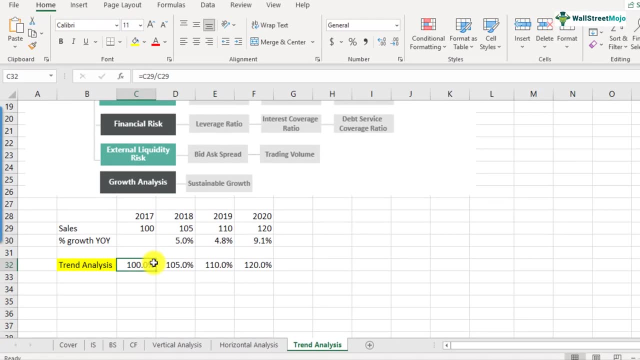 over the years, but the base year remains the same. in trend analysis, Usually this is shown by way of a graph and it's very helpful, So I'll just quickly create a graph as well. A 2D graph would be very helpful. 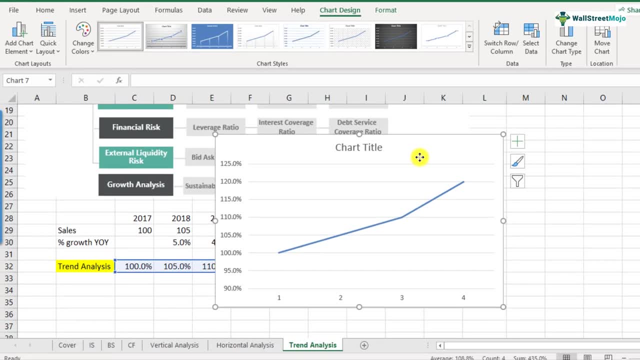 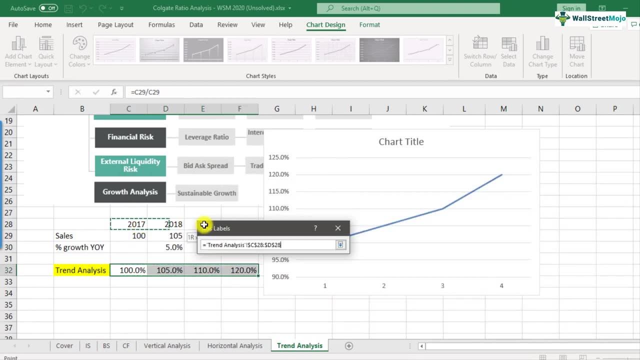 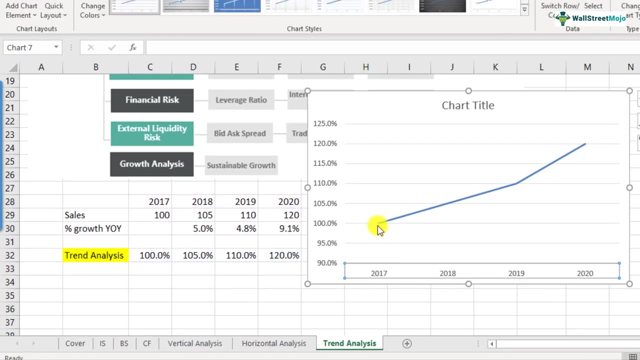 You can go to this 2D line charts and see that. Okay, You can just change the year as well. Years from 2017 to 2008.. Okay, Now you can see for 2017, obviously it's a hundred percent. that's the base year. 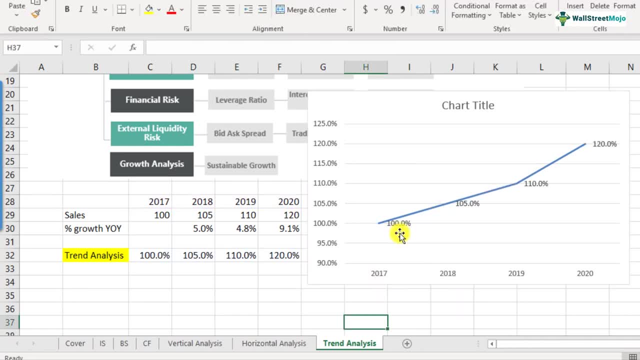 But from that year onwards things have changed from a hundred percent to 105%. That would mean 5% growth in one year's time. 110 means 10% growth in two years time, And likewise we have 120% here. 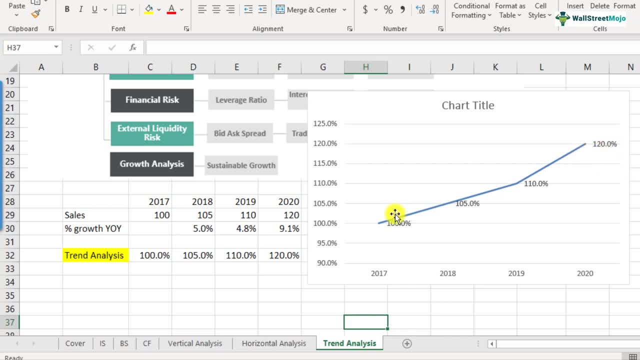 That means 20% growth over a three year time frame. So that's how trend analysis is kind of interpreted. So let's now look at our Colgate case study and make the trend analysis for the same. So here is the income statement of Colgate PowerLive. 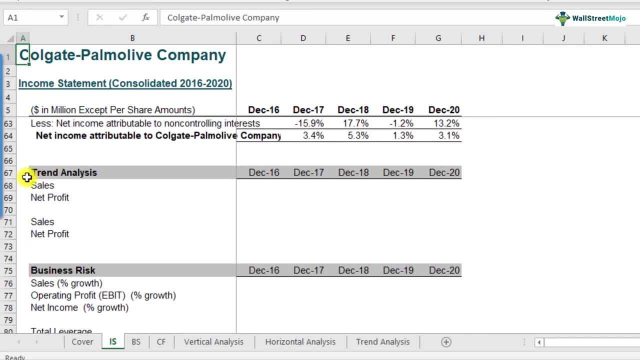 And why don't you scroll down to the trend analysis section, which is at row number 67.. Here we'll be doing trend analysis only on two line items, That's the sales and the net profit, But you can actually do it for all the line items. 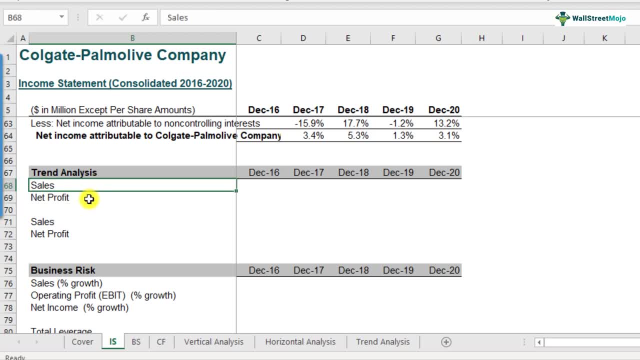 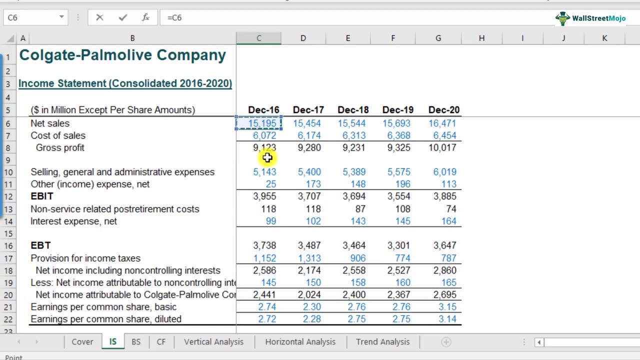 That should not be a very big issue. I, just for the sake of convenience, have taken only two data points: Okay, Sales and net profit. So the first step is to link the data items from the respective income statement. I'm linking the sales from December 16.. 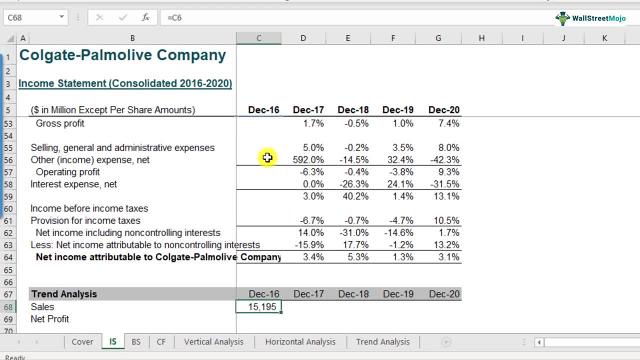 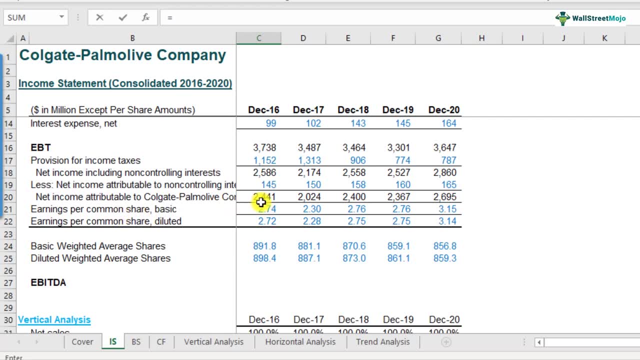 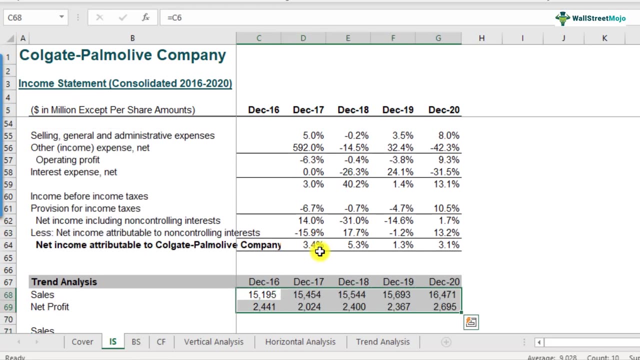 That's 15195.. So I'm just linking it here. No rocket science. Net profit, It is nothing but your net income. Net income is 2441.. Okay, For December 16 year: Okay, So I've just taken and linked these respective years data and I'll be doing the trend analysis. 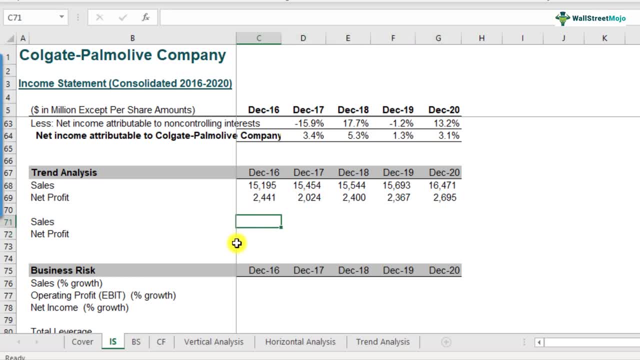 in this area. All right, So let's do that. The first step, as I said earlier, was to divide this base year by itself, So that gives us a hundred percent. And then for the next year divided by the base year, right? 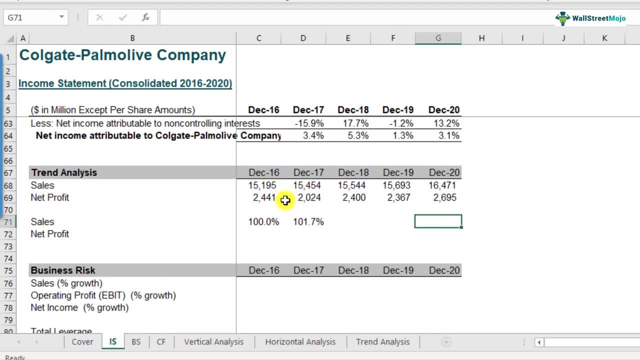 So that's. that's what we keep on doing. If there is lots of data, it will be very cumbersome for you to keep on typing the formula, So in this case you can use an absolute reference. The absolute reference means this cell C28 won't change. 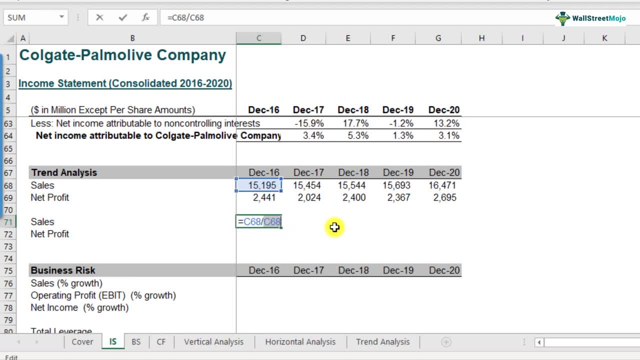 That's what we want. There's a shortcut to ensuring that formula doesn't change. That's called as absolute reference And you can click on F4.. Press F4. And there are two dollar signs that we get added. This is called as absolute reference. 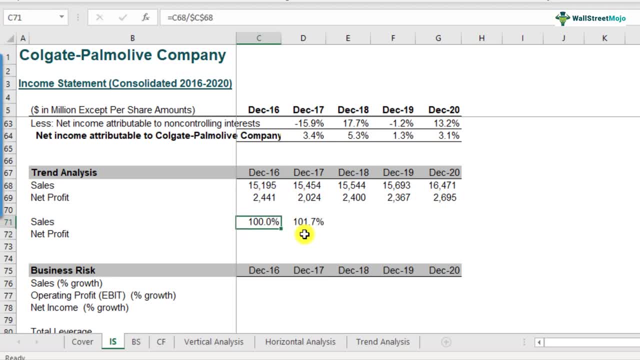 Once you do this minor change in your formula and you can copy and paste your formulas you know across the rows, That's how it works- The base won't change at all. Likewise, you can do the same for your net profit. 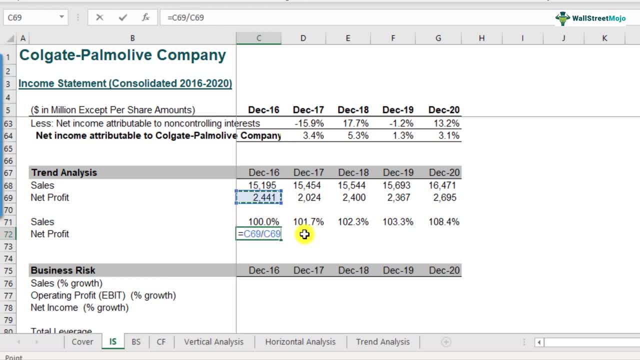 So net profit: is this divided by this? And obviously I'll do. I'll press F4. So that it becomes an absolute reference. The base doesn't change and you can copy and paste it across, All right. So this is how you can actually go about doing it. 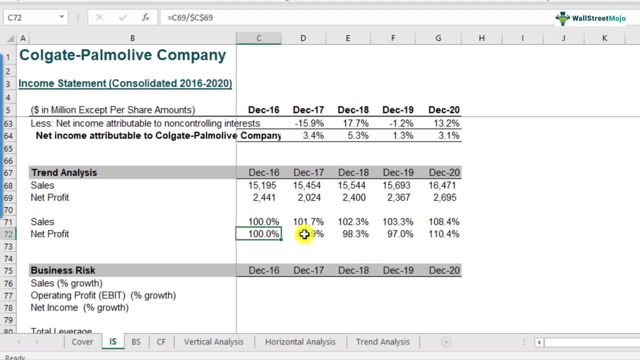 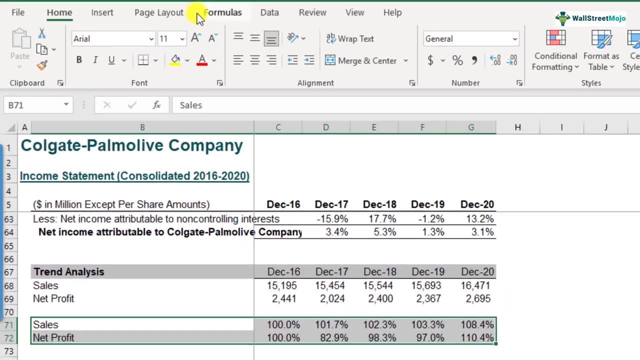 And obviously for trend analysis. as I said, it's easier to visualize it via a graph, So you can do that as well. You can probably, you know- copy and paste this data in the graph like this: Let's say: this is the data point. 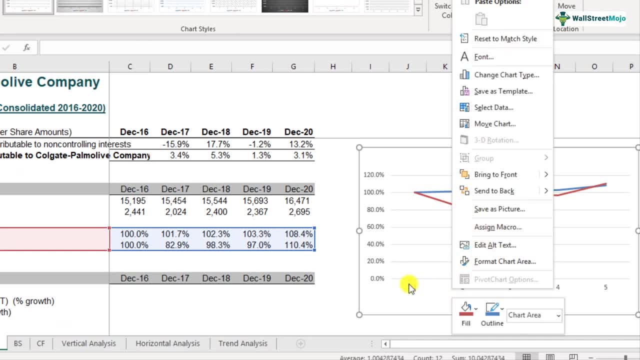 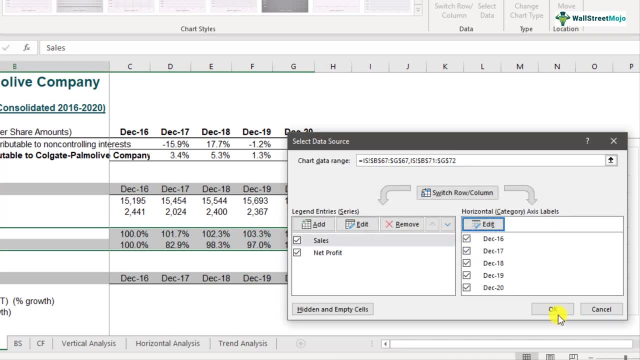 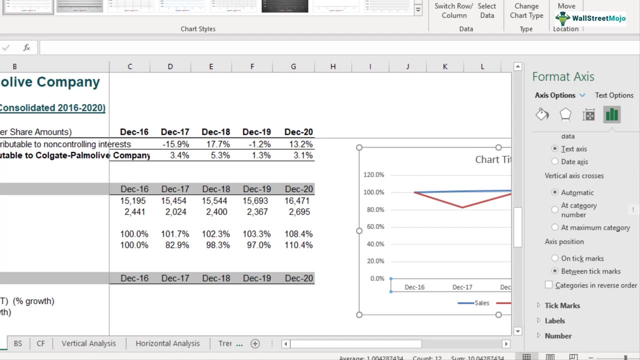 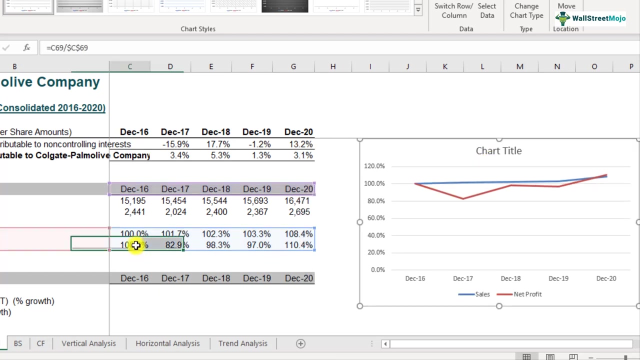 And you can change the year as well. Okay, Let me change the year. Okay, My taxes. I think this should work. So, as you can see, here we can see a specific trend. The trends here are like you know, the net profit was a hundred percent, but it suddenly 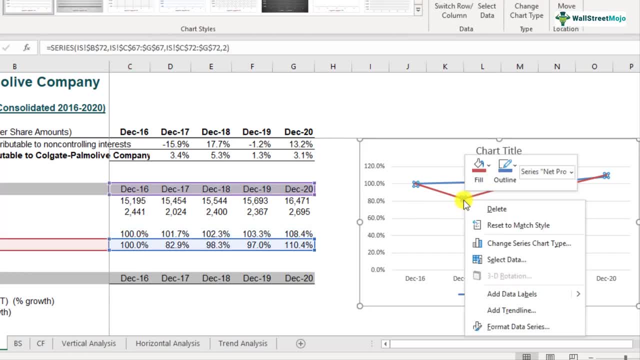 dipped and it is kind of visually Seen here Right. If I add the labels you will find it was becoming. it became 82.9% here, 98.3%, 97 and 110.4%, So the trend in net profit has been kind of a bit volatile.